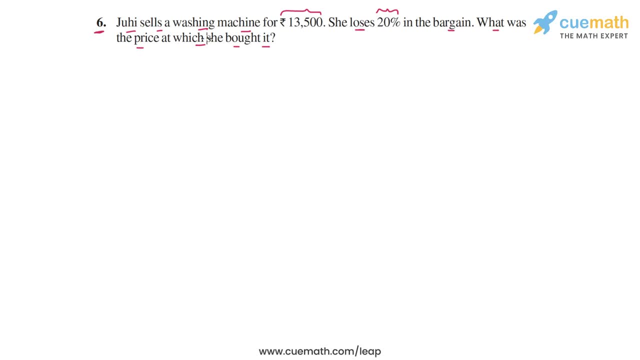 is unknown, But we do know that Juhi sold the machine for Rs 13,500 and made a loss of 20% on this sale, And we have to find the cost price using this information. Okay, so let me show you two slightly different approaches of solving this problem. Okay, so our first. 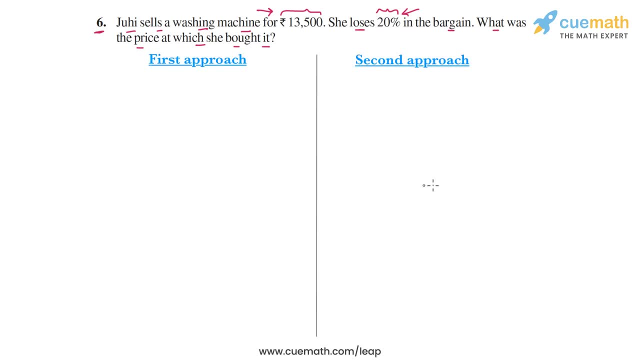 approach is going to be based on the unitary method. Let's see how we can apply the unitary method in this case. So we are given that a loss of 20% was made correct. This means that if the cost price is, let's say, Rs 100, then the loss will be how much? If the loss 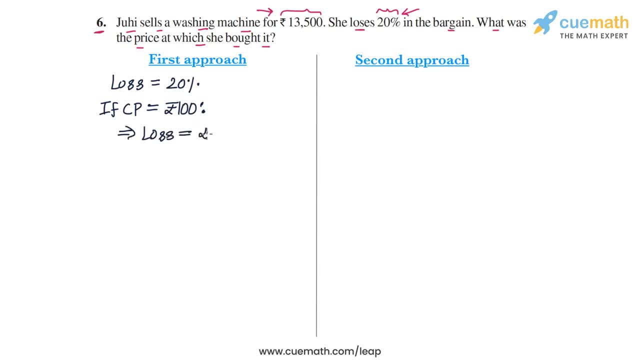 is 20%. so on a cost price of Rs 100, the loss will be Rs 20.. Next, the selling price in this case will be the cost price minus the loss, or Rs 100 minus Rs 20, which is equal to Rs 80.. So what we have basically done so far is for: 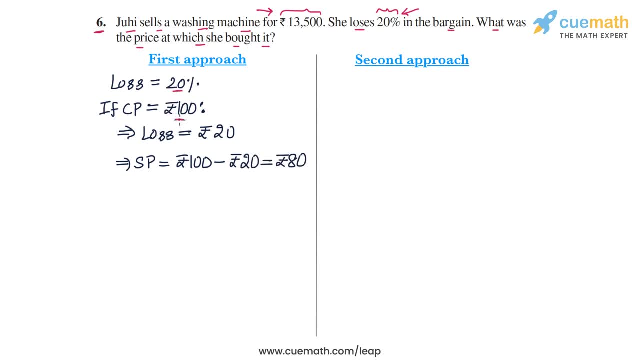 a loss of 20%. we have seen that a cost price of Rs 100 means a selling price of Rs 80. So let's write it this way: A selling price of Rs 80 corresponds to a cost price of Rs. 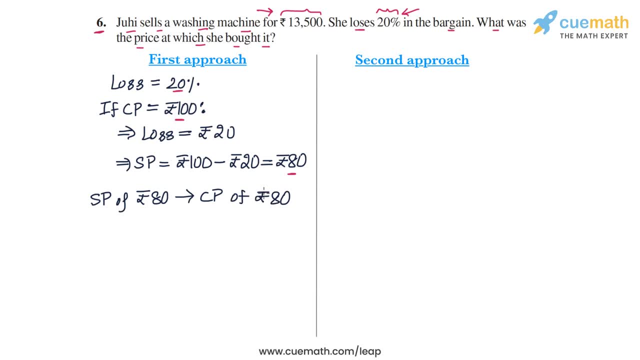 100.. Okay, so selling price of Rs 80 corresponds to cost price of Rs 100.. Therefore, if the selling price is the actual selling price, which is Rs 13,500.. So if the selling price is Rs 13,500, now we apply the unitary method. Now we can calculate the cost price, The 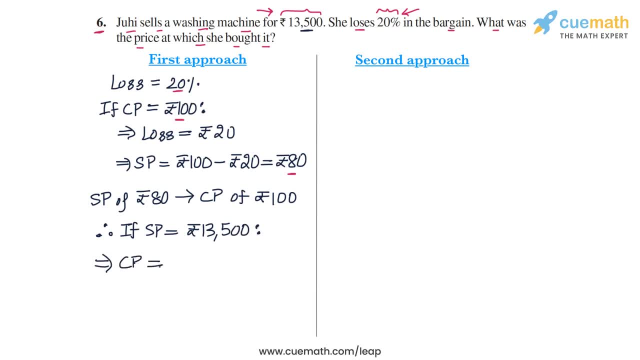 cost price will be: Okay, We will take 100 by 80 and multiply it by 13,500. So the cost price will be Rs 100 divided by Rs 80 into Rs 13,500.. So this will be the cost price. And now we simply. 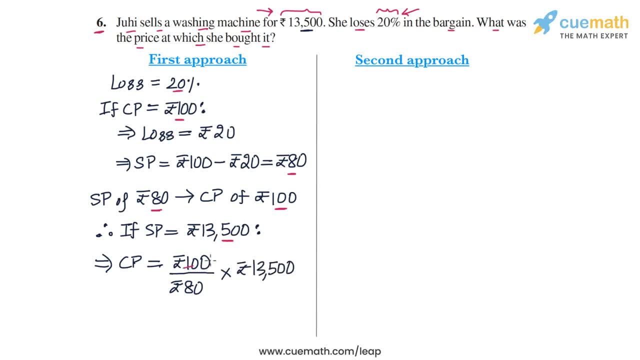 have to calculate this product. So 100 by 80 is 5 by 4, and then 5 into 13,500 is 67,500, which, when we divide by 4. We will get 16,875.. Okay, so 16,875.. These many rupees. So this is the cost price, Okay. 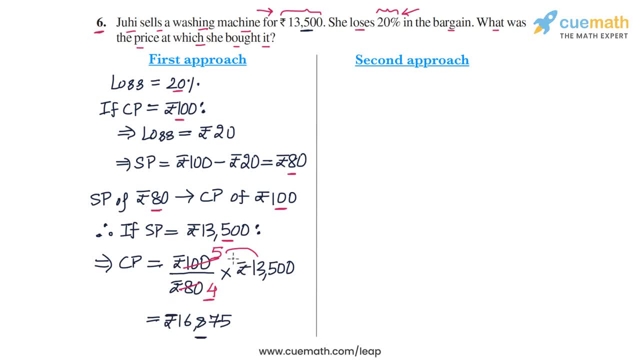 Now for our second approach. we will set up an equation in the unknown, which is the cost price of the washing machine. Let's see how to do this. So, once again, we start with the information that the loss is 20%. Okay, And let's assume that the cost price, which 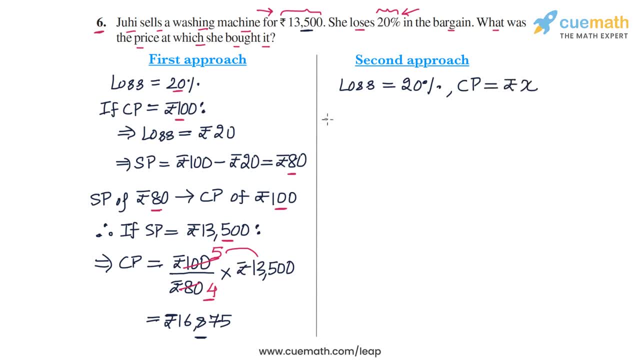 we have to find That is Rs X. So now we calculate the loss as 20% of X, So we calculate the loss in terms of X. So the loss will be 20 by 100 of Rs X, So 20 by 100 into Rs X, Now 20. 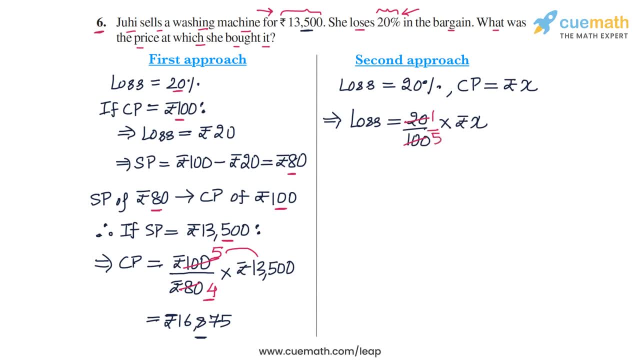 by 100 is 1 by 5.. So 1 by 5 into Rs X is Rs X by 5.. So this is the value of the loss. Okay, Okay, So this is the selling price. So the selling price will be the cost price minus the loss. 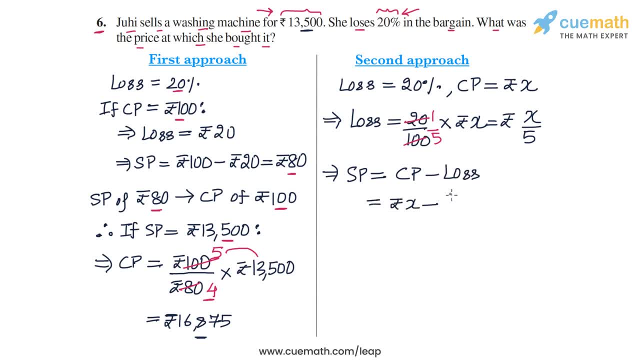 And the cost price is Rs X, The selling price, the loss, is Rs X by 5.. So we are subtracting from Rs X, We are subtracting Rs X by 5. And that will give us Rs 4X by 5.. Okay, Because. 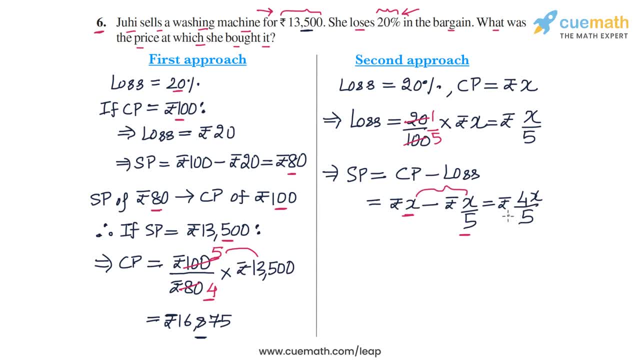 X minus X by 5 will be 4X by 5.. Okay, So 4X by 5.. But we also know that the selling price is Rs 13,500.. So we are given that the selling price is Rs 13,500.. So what this means is basically that we can equate. 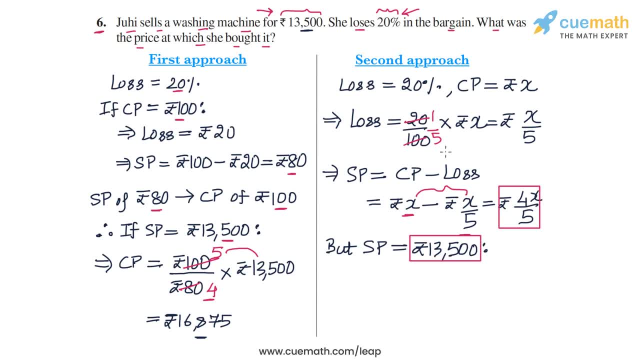 this expression with this value, and that will give us the value of X. Okay, So let's do that. So 4X by 5 will be equal to 13,500.. Okay, So 4X by 5 will be equal to 13,500. And therefore X will be equal to. So we take 5 into the.